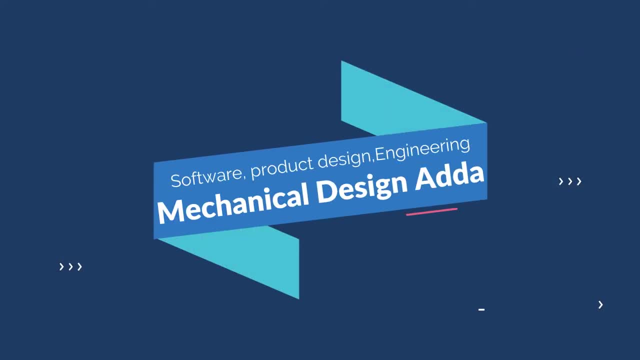 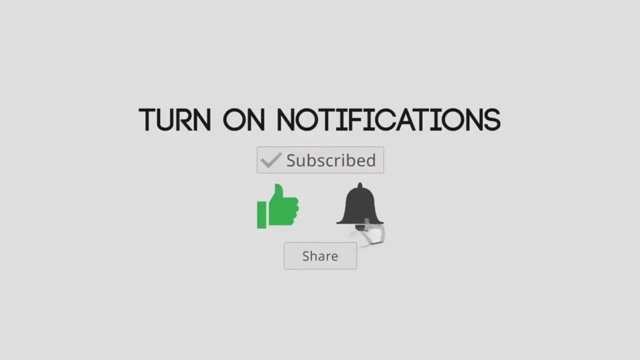 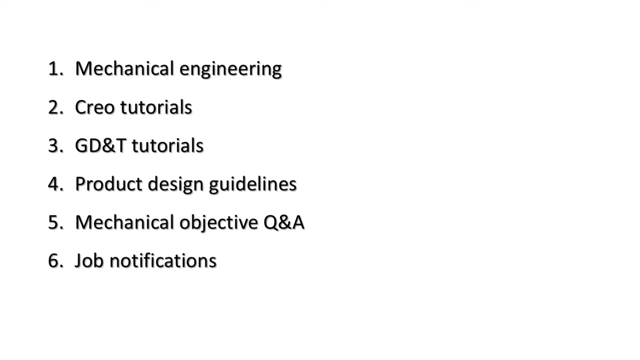 Hello friend, welcome to my YouTube channel, Mechanical Design Adam. In this video we will discuss some design guidelines of sand casting. If you are new here, subscribe the channel and hit the bell icon Because we upload the videos on mechanical engineering: Creo tutorials, GD&T tutorials, product design guidelines, mechanical objective questions for the government exam, job notification and previous year solved question papers for the mechanical engineering. 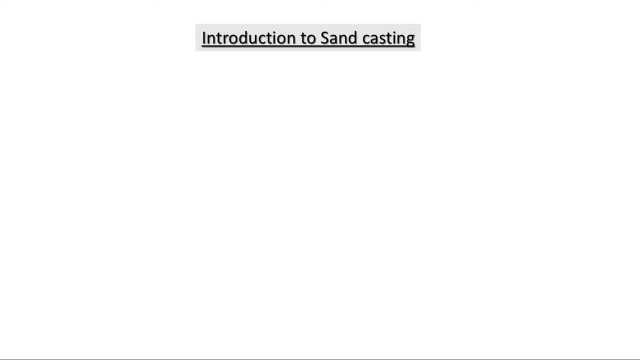 So, friend, before going to discuss the design guidelines of sand casting, let's quickly understand what is sand casting, its process, applications, and advantages and disadvantages. Sand casting is a widely used process in which we pour the molten metal into the cavity of desired shape and allow to solidify to get a desired product or casting. 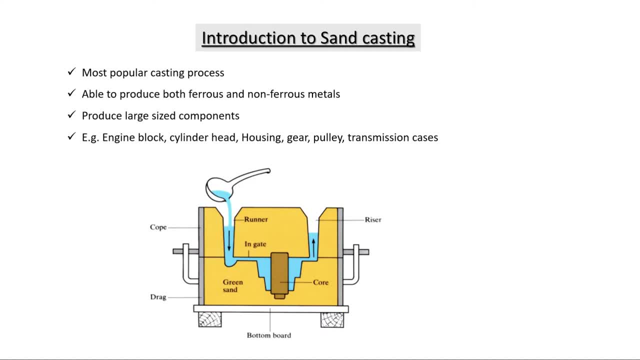 And sand casting is used to produce very large and complex shapes. So, as you can see in the picture, there are some parameters like runner, gate, riser, scope and drag, like this, and the core. The core is generally made up of the sand. 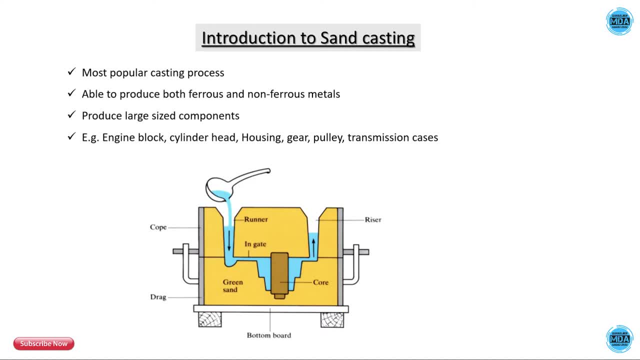 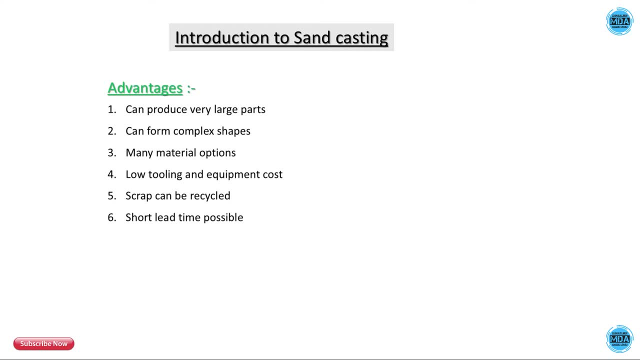 So after the solidification we break the mold and the core. Some advantages of sand casting: it can produce very large components and complex shapes And many materials options. like we can produce is with the ferrous material and the non-ferrous material. 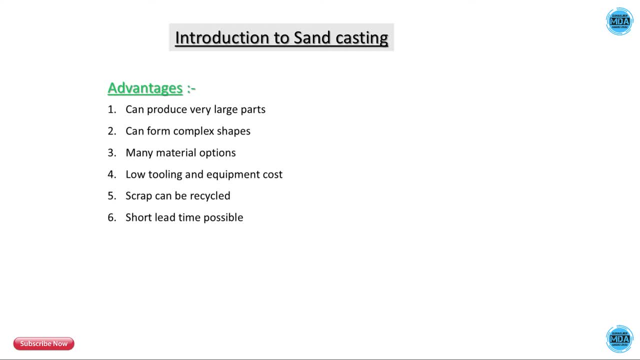 This crap can be recycled. So here the mold is made up of the sand, so we can reuse with some additives and the short lead time is possible here. And the disadvantage of the sand casting is poor material strength, high porosity possible for surface finish and total secondary machine operations is required, low production rate. 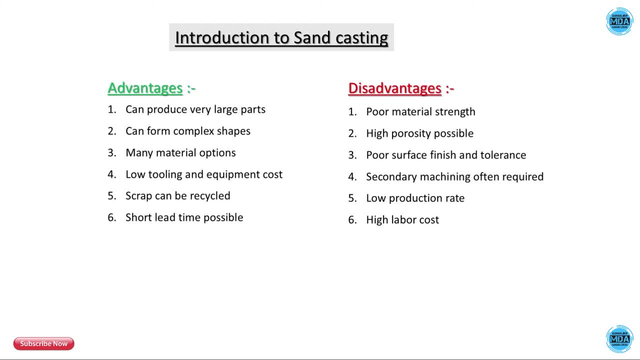 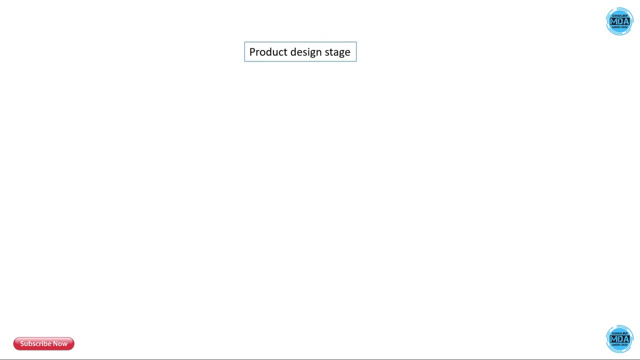 and the high labor cost here. the skilled person plays very important role here. so the sand casting is a very long process, like firstly we have the product design stage and then the molded design stage, in that we design the runner, screw gate patterns like this, and then the foundry work. 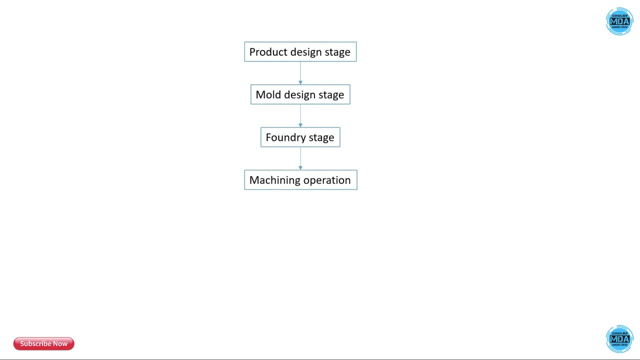 in the foundry work, the operator skill plays very important role. and then for the secondary operation or the post operation, the machining work and then the inspection work, and after that we get the finished casted component. in this video we will focus only on the product design stage. 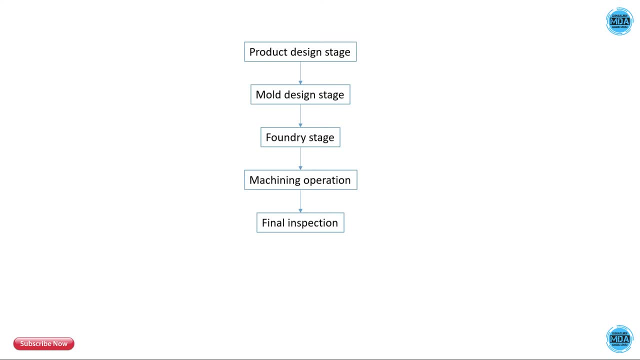 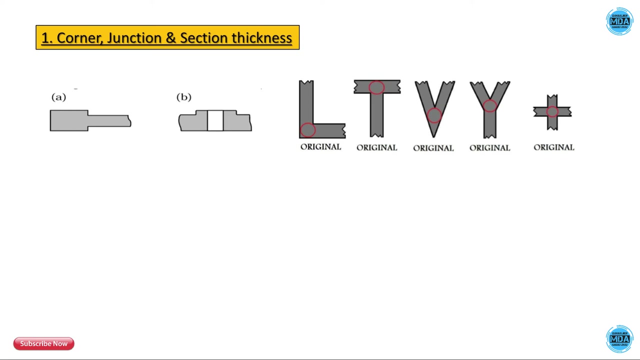 so while working on the casting component, the designer should follow the guidelines so that we can provide the good quality of casting that can be final product. so let's discuss one by one. first guideline is corner junction and sectional thickness. the sharp corner and the angle they can produce the high stresses in the casting that may cause the cracking and tearing. 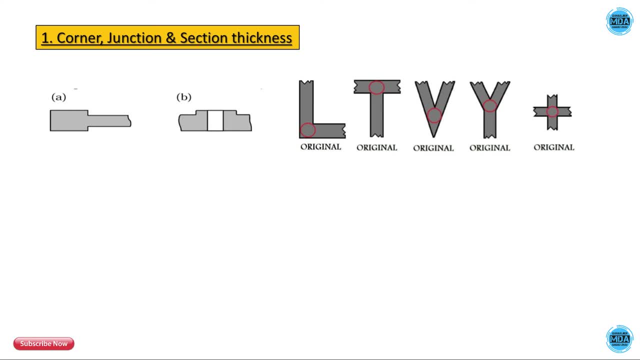 of tearing of the casting during the solidification. and next one is the junction. if the two sections are two or more sections are combined at a one point or intersect at a one point, they form a junction. so at that intersect point the material is more so. the junction like l, junction t, v, y, x, like. 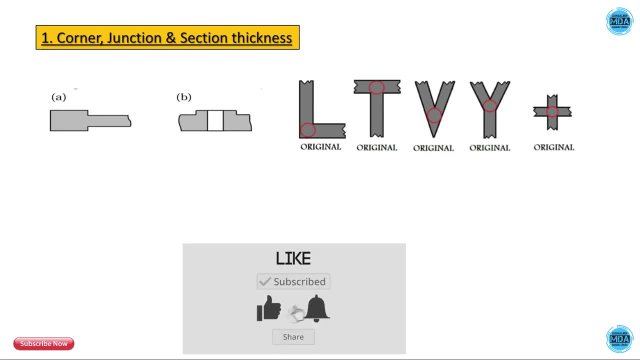 this. these are the type of the junctions at that time. there is no uniform thickness when the junction is formed, so the sudden drop of section is not desirable for the process. because of the corners junction and the sudden drop of the section there are some problems created during the casting, like 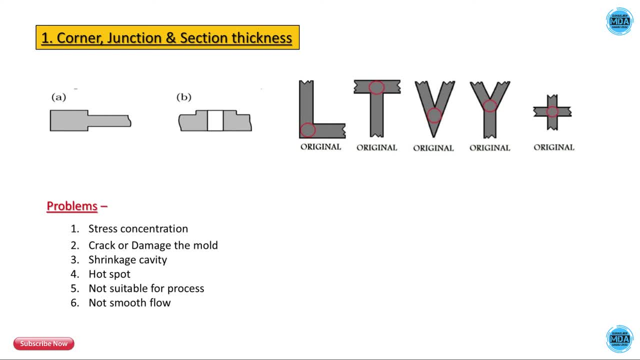 stress concentration, damaging of the mold, shrinkage cavity and the hot spot may created and the sudden drop of the section is not suitable for the sand casting process because because it may break the mold and there is no smooth flow for the sudden dropping to avoid the sharp corner, we 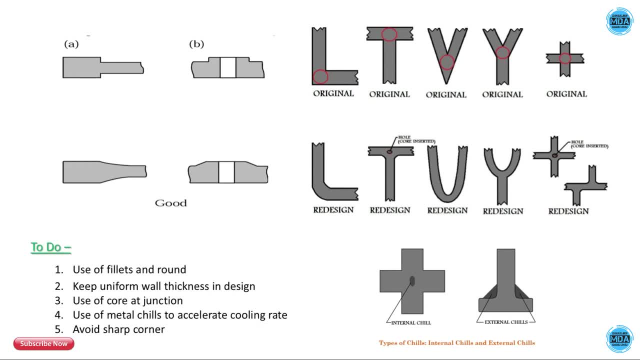 using the fillet and the round. so so minimum 3 mm fillet, three fillet we can use and and keep the uniform wall thickness in the design. if you are casting having the junction, then redesign the junction, or if you want an uneven thickness, then or this one is your requirement, then at that time 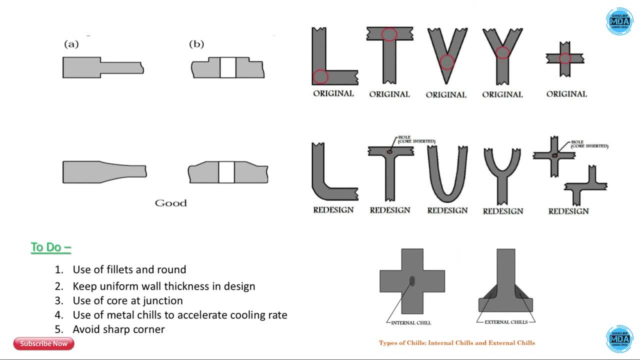 you can use the core at the top and at the bottom if you want to use the main connection, also for a at the junction or metal shield at the junction, because we know that during the solidification the cooling is from outer side to inner side. so because of the outer shrinkage the 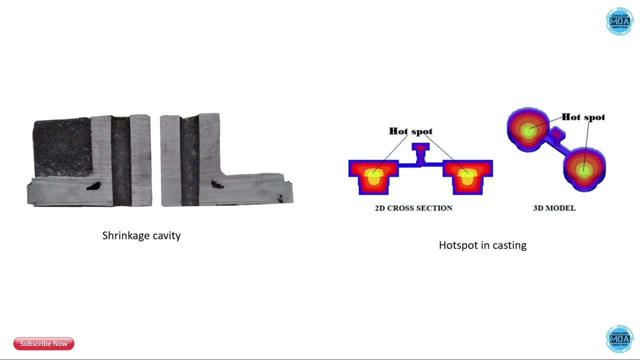 internal cavity is created because of the outer portion is shrink, the inner portion created the cavity. and the cavity created because of the shrinkage is called as the shrinkage cavity. and next one is the hot spot: the cooling of the outer section and the inner section remains hot. 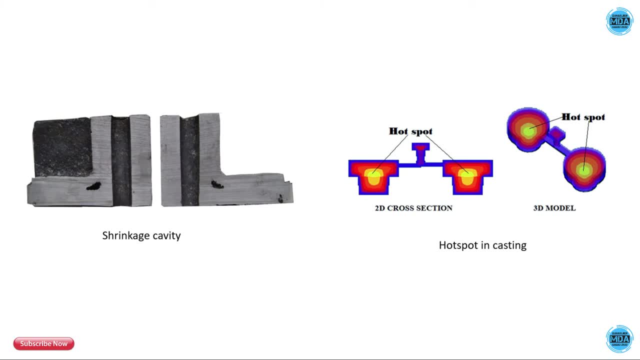 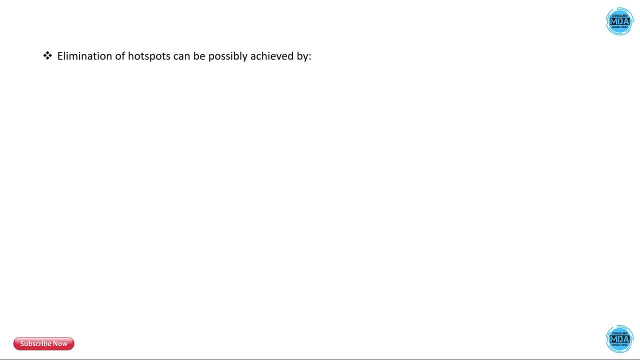 that defect is called as hot spot. the inner portion is remains hot because the cooling cycle is completed, but the inner portion is not cool because of the thick section. so the hot spot hot spot can be avoided by adding the core at the thickened section, by feeding the molten metal through the riser or redesigning the junction. like this we can avoid the 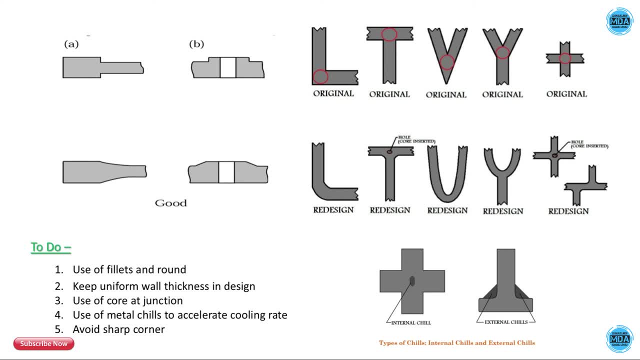 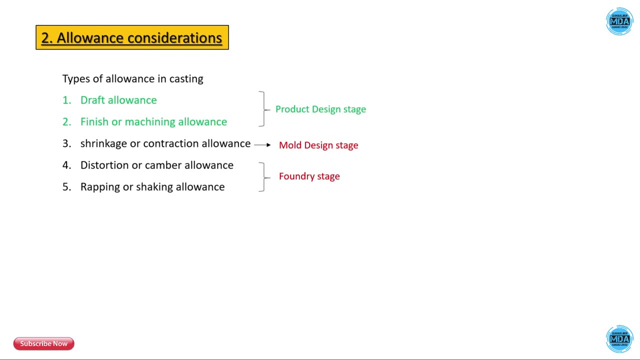 hot spot. we can use the metal cheese to accelerate the cooling from inside or from the external. we can use the chill to accelerate the cooling. next one is that allowance consideration in the casting. so there are different types of allowances, like draft allowance, machining allowance, shrinkage allowance. 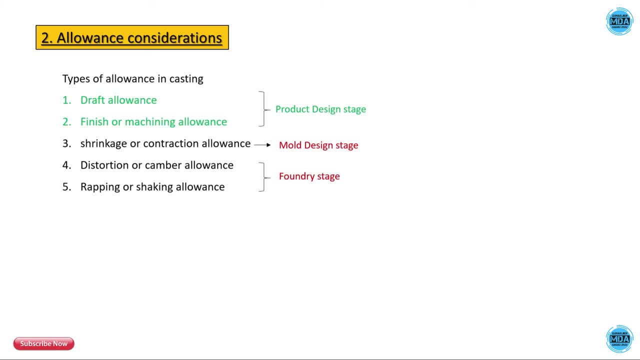 distortion allowance, wrapping allowance or the shaking allowance. so these are the five types of allowances. at the design stage we consider only two allowances, that is, draft allowance and the machining allowance. so in the shrinkage allowance it it is considered in the mold design stage. so and the remaining, remaining distortion and the shaking allowance, these are considered in. 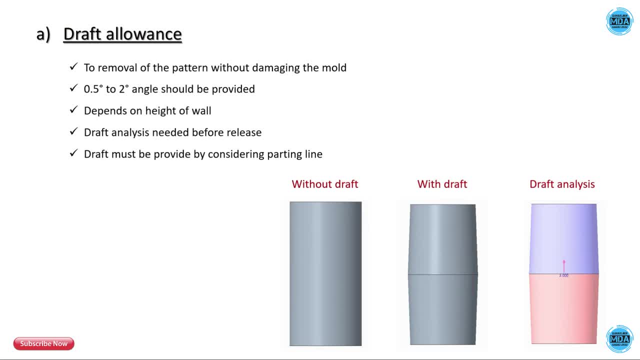 the foundry stage. so we will discuss the draft allowance first. so to remove the pattern from the mold, the draft is required. so we are applying the draft or angle to the vertical, to the all vertical surfaces of the casting so that we can easily remove the pattern from the mold to two degree. 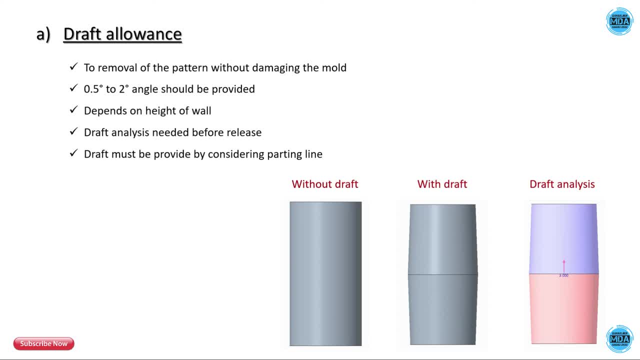 we can apply the draft to remove the pattern. but you can use as per your requirement, because the draft is depends on the height of the vertical surfaces. as you can apply the suppose you have the height of, suppose you have the small height, at that time you can apply the larger angle. if you have the larger height, then at that time 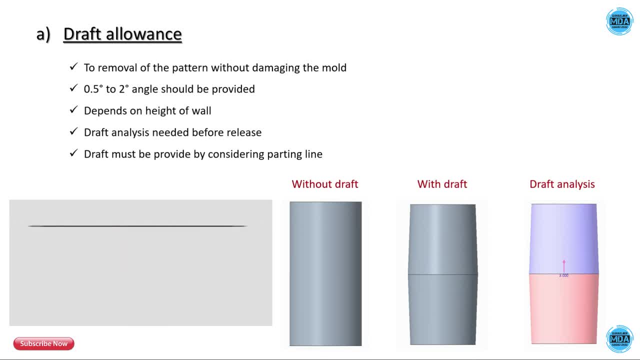 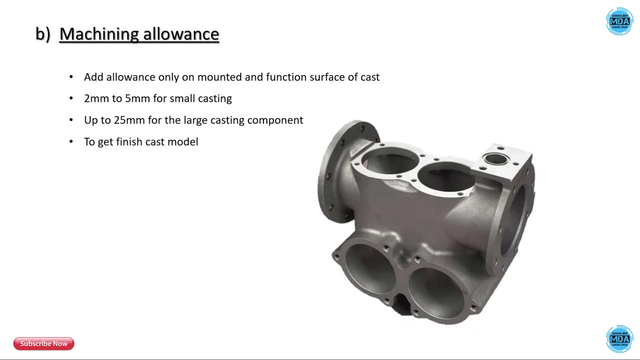 the smaller draft angle must be applied. be there, because if you apply at the large angle to the large height, then at the bottom, at the bottom, the material will be more. the draft angle is inversely proportional to the height of the vertical surface of the casting. next one is the machine allowance. so machine allowance. 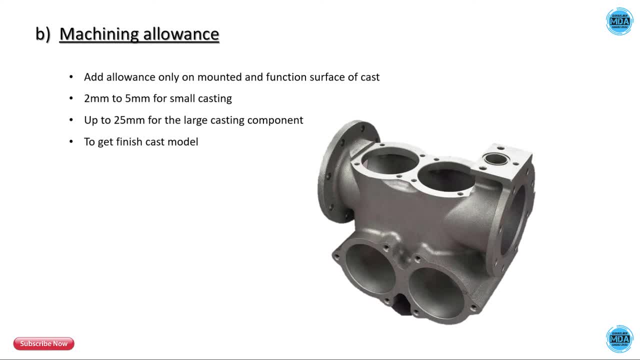 it is a post operation where we remove the material for the mounting for the mating surfaces like this. the requirement of the surfaces we machine generally the 2 mm to 5 mm machining allowance must be provided at the design stage only and this must be provided on the mounting. 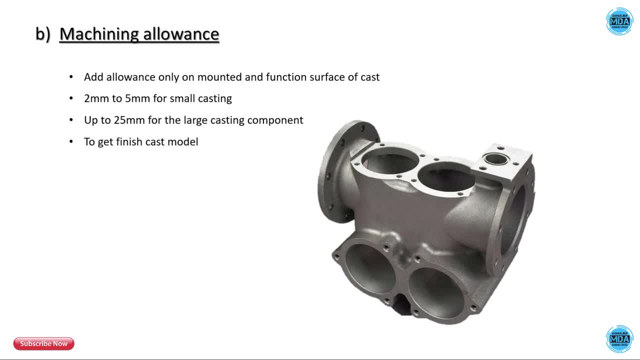 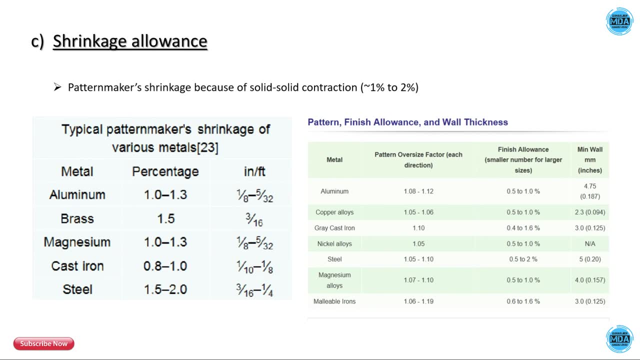 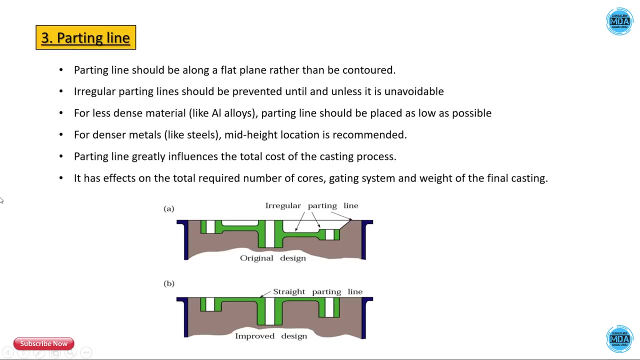 surfaces or the mating surfaces only. as you can see here, the shrinkage allowance, machining allowance and the wall thickness data are given here for your reference purpose. next one: we have the parting line. so the parting line plays very important role because the determining the position of the 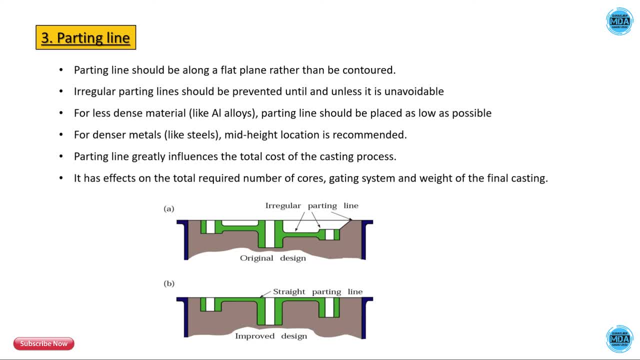 parting line is the critical step in the casting design because its effects on the cost number of core gating system and the weight of the motive system of the gating system also depends on the. the final casting parting line should be flat rather than the counter, so it must be flat along. 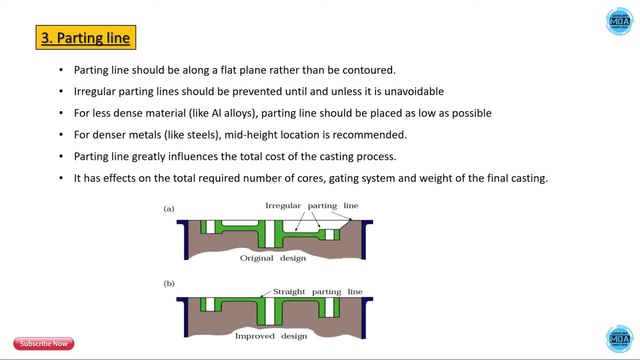 so that the mold mold creation will be easy. if it is irregular parting line, then the complex mold design will be there and for the dense material, like aluminum alloy, the parting line should be placed as low as possible and for the denser material, like a steel, the mid-height